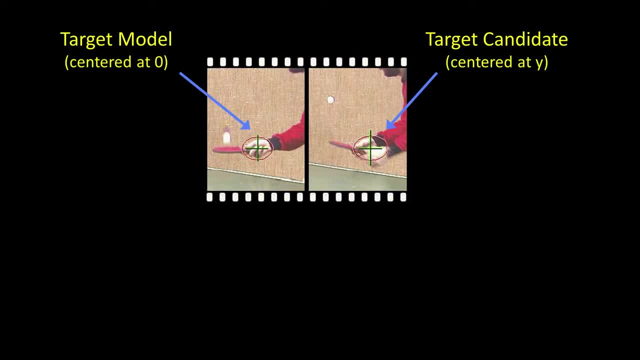 Okay, so here we have two frames. On the left we have the original model, The. the model is sort of a time and and we're going to call that zero, And on the right we have some candidate, something. 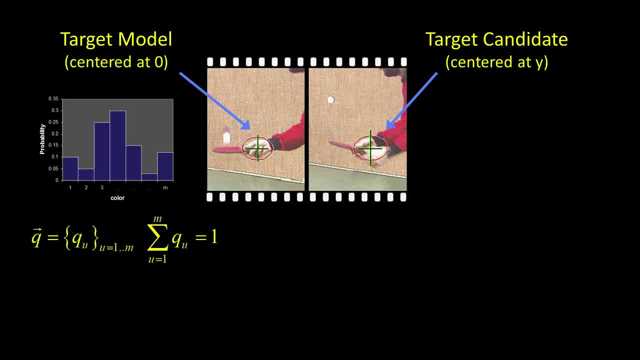 some place in terms of how it's changed, And it's going to be centered at some value y, some pixel y. So on the left we have our initial distribution. Okay, so this was our histogram that we computed in our area. 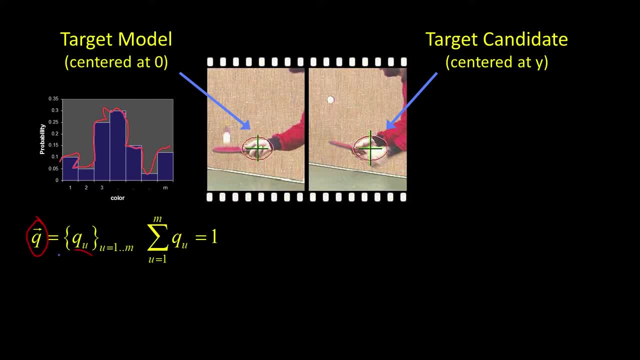 And it's typically called q, And q's got a set of bins- u, 1 through m, And because it's going to represent a density, we enforce the fact that the sum of them equals 1.. So how do we do that? 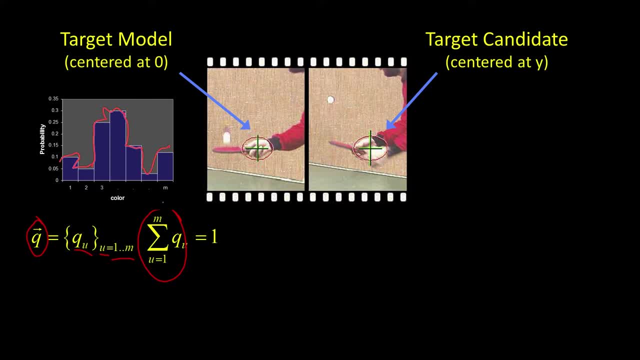 Well, we just sum them all up and we divide all the bins by that value. Okay, and you see, we have the audaciousness to call it probability. Okay, because well, we're going to take these samples and we'll assume that it's representative of a probability distribution function. 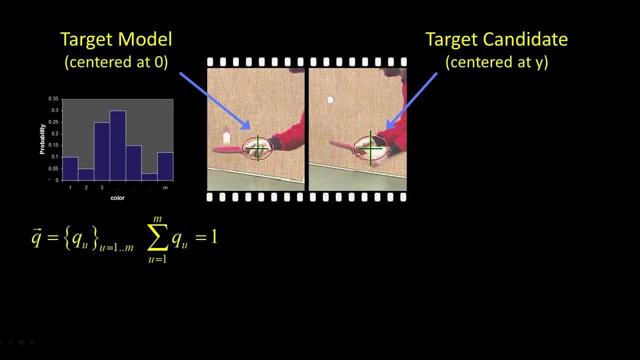 So that's our distribution at the initial of the target. At some new location, okay, we can compute the distribution again. So now, p of u is a function of y, where y is the point that we're considering. Remember you have to consider p of z, given the state. 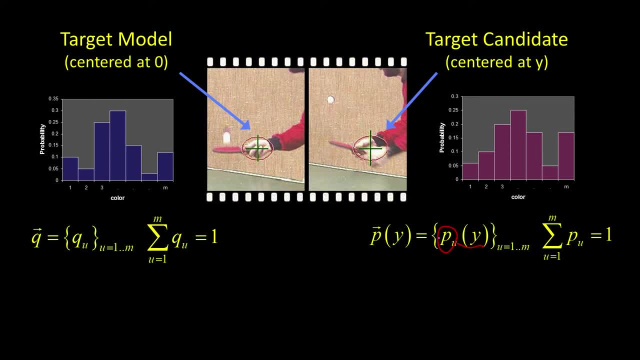 So y is going to be that, that new point, And I it's called y instead of x. That's how it's done in the mean shift literature. If you read this, this is this is what you would see. And again, we're going to build a distribution. 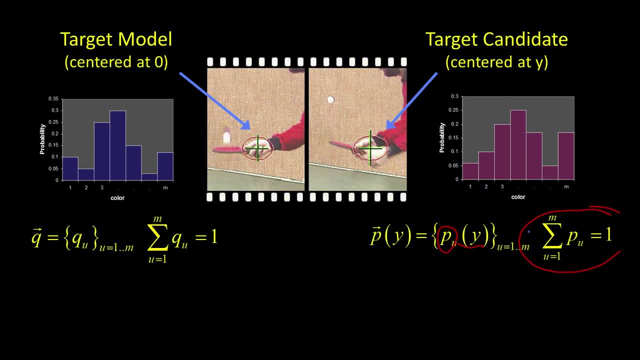 by assuming that these things sum up to 1.. So we have these two distributions And what we have to do is we need a similarity function that compares them, that compares the original q and the new p of y, which is the density at this proposed place. 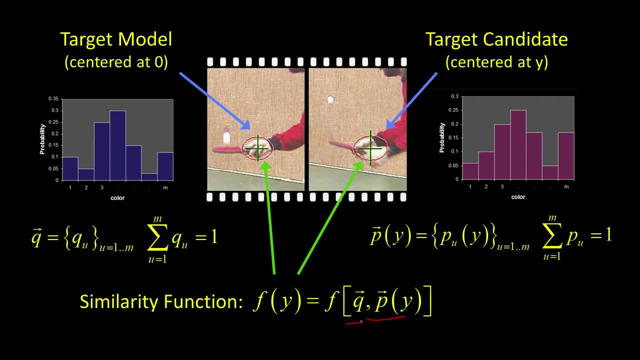 So the question is: how are we going to compare these distributions? Now, there are a variety of functions that you can use to compare histograms. where the histograms are are normalized to 1, so they represent probabilities. There's the min value. 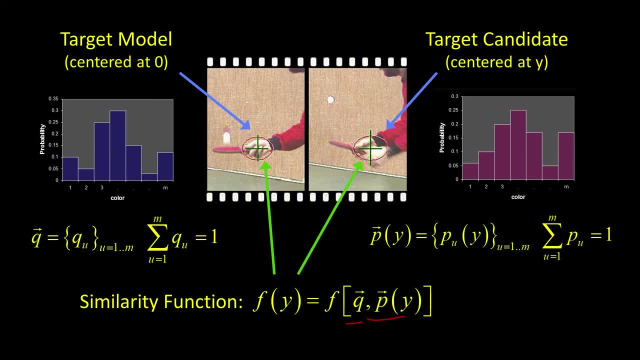 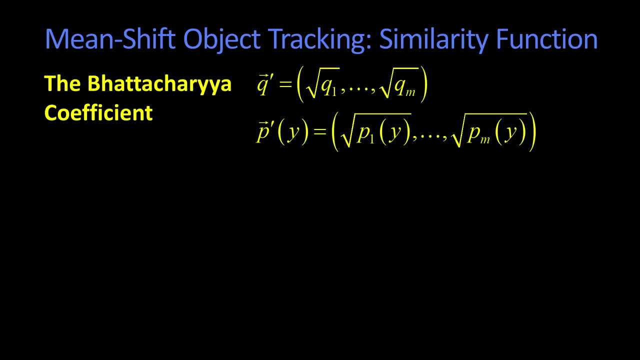 There's, there's chi squared. There's a variety of them. The one that was used with respect to mean shift tracking is referred to as the Botticelli coefficient. Botticelli coefficient comes from something related to the Botticelli distance. 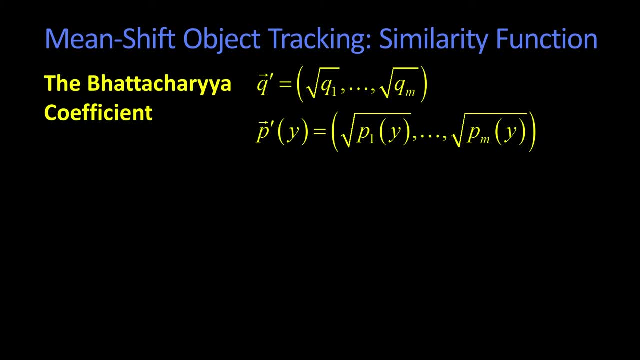 It's simply a way of comparing distributions. What you do is you take your distributions here and you change it by taking the square root of each of the components. So if q is a distribution, q1 through qm, then q prime is going to be square root of q1 through the square root of qm.